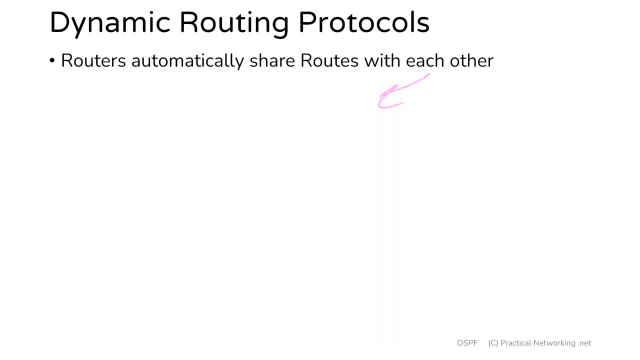 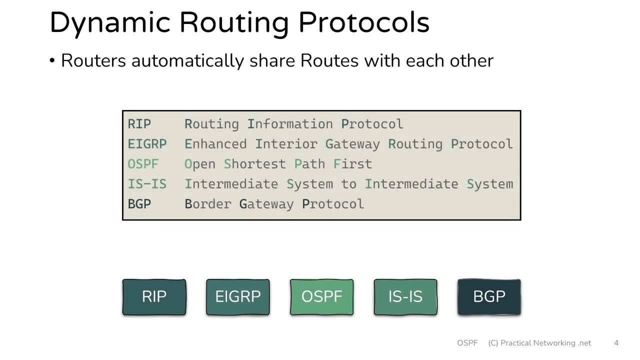 the last thing I told you on this particular slide is that there are five major dynamic routing protocols that exist, and each of them differ insofar as how they detect other routers participating in the same dynamic routing protocol and what they share, when they're actually sharing routes with. 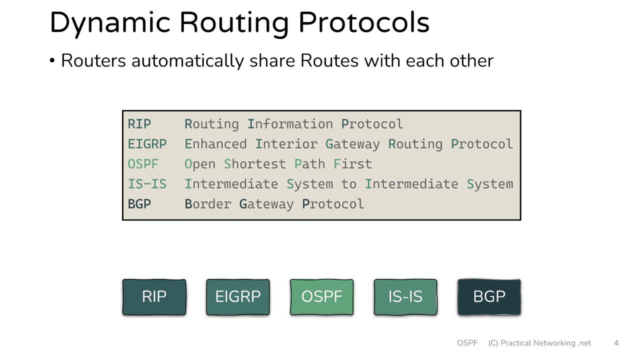 one another. Now, the inner workings of each of these are pretty fascinating, but we're not going to go into too much detail about that in this video. So let's get started. The first category that we're going to discuss is the concept of IGPs and EGPs. 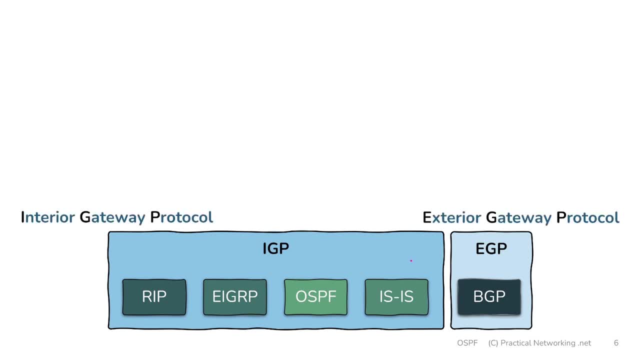 IGP stands for Interior Gateway Protocol, and they include RIP, EIGRP, OSPF and ISIS. EGP stands for Exterior Gateway Protocol, and the only EGP in use on the internet today is EGP, the Border Gateway Protocol. 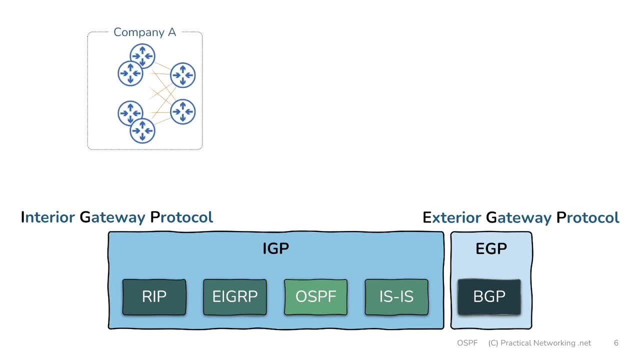 Now to discuss these concepts. we're going to use these two company networks. Since these are two separate company networks, they can each be referred to as an autonomous system. Now, the concept of an autonomous system is very important, so I do want to give you a 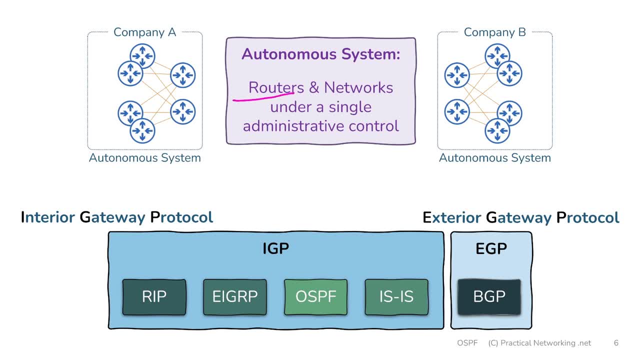 formal definition, An autonomous system is any set of routers or networks underneath a single administrative control. Since this is a different company network than this, each of these are referred to as their own autonomous system. With that in mind, we can now explore what an IGP is. An IGP is best suited for sharing routes within a particular autonomous 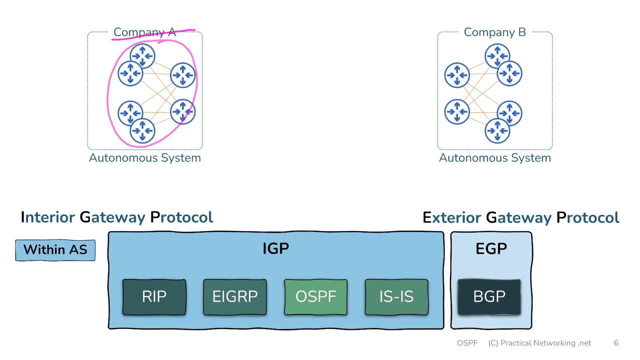 system, Meaning these routers over here belonging to company A might be using EIGRP to talk amongst themselves and share the networks that exist inside company A, And these routers over here belonging to company B might be using OSPF amongst themselves to talk and share routes. 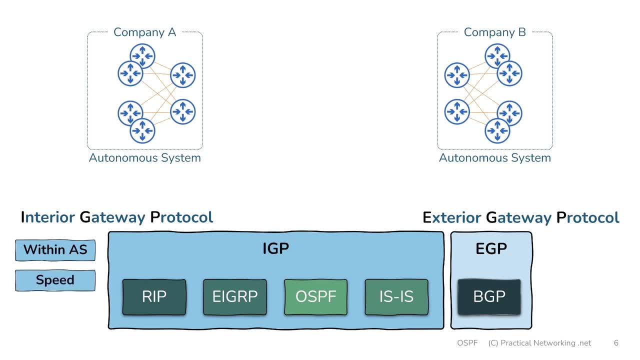 with one another. IGPs are typically tuned for speed and responsiveness happen to that router right there. we would want the other routers in the topology to instantly know that some sort of failure event has happened and then adjust their routes accordingly. To do this, these IGPs tend to be pretty chatty, but that's what you pay to get this additional speed. 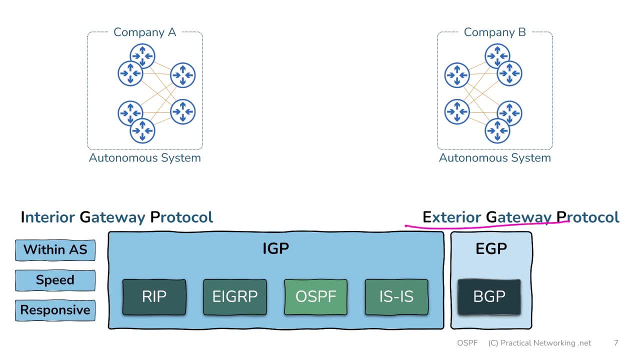 and responsiveness By comparison. exterior gateway protocols are built for sharing routes between autonomous systems, meaning company A could share with company B the IP address space that company A owns, and company B could then do the same. Now, typically companies aren't so big. 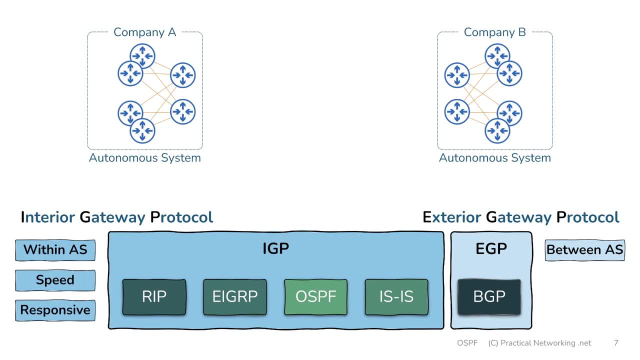 that they share IP address space with another directly. Some companies are that big, but most companies will share their routes with an ISP or an Internet Service Provider. Each company is connected to one or more Internet Service Provider and then those companies will share their routes with those particular Internet Service Providers. 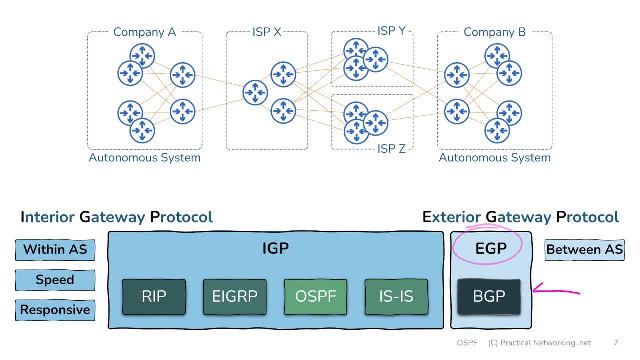 and they'll do that using an exterior gateway protocol or mainly BGP. These interconnected ISPs are essentially what the Internet is: It's just a bunch of Internet Service Providers that are all connected to one another. Either way, each of these ISPs are their. 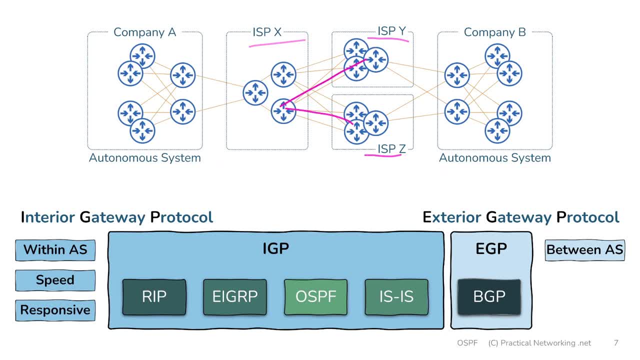 own autonomous system and each of these ISPs will share routes with each other and different companies using something like BGP. Unlike IGPs, EGPs are tuned for stability, meaning again, if something were to happen to that router, company A might want all the other routers in this topology. 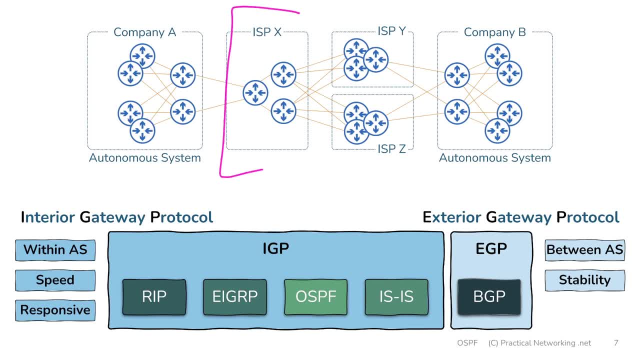 instantly know about, But we might want to shield the rest of the Internet from knowing. something small occurred in company A's network. If you think about it, how many different failures occur in all the thousands of companies that exist out on the Internet? We wouldn't want the 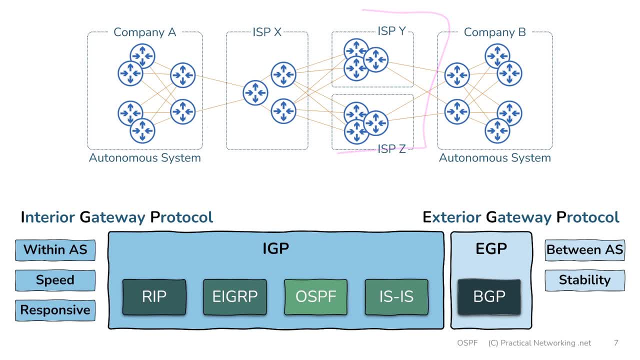 entire Internet to be flooded with every single small failure event. Instead, exterior gateway protocols will limit intentionally how often updates are sent or received. Moreover, exterior gateway protocols are also tuned for security and control. For instance, with BGP, this ISP might know the IP address space that company A owns. 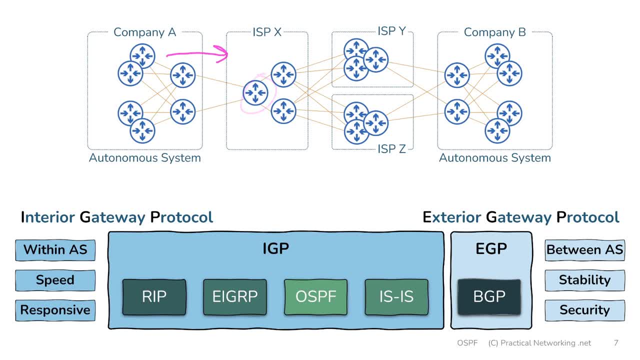 and might tell this router that it's only going to accept routing advertisements from company A that belong to that particular IP address space If company A decided to start doing something malicious and advertise out into the Internet that it actually owned company B's IP address space. 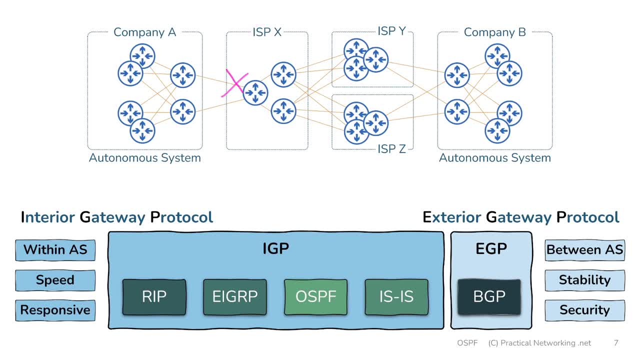 this Internet Service Provider would know about it and would reject these routes. Now some IGPs do have methods of filtering routes, but not nearly the degree that an exterior gateway protocol like BGP does. Moreover, BGP gives company B the ability to share routes with ISP Y and ISP Z. 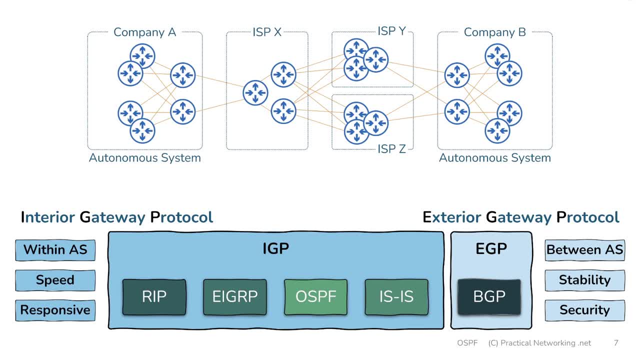 but also include information and preferences which can influence the rest of the Internet and how they choose paths to get to company B's network. Maybe company B wants to prioritize traffic going through this path because this link is faster or is less expensive service With an exterior gateway protocol like BGP. 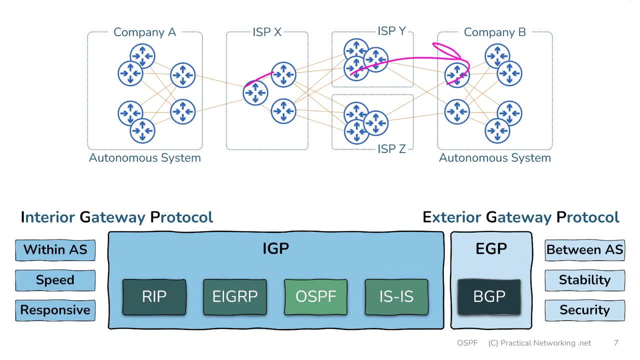 you can influence the route selection of ISPs, multiple autonomous systems, away. In fact, BGP has a whole 12-step route preference sequence it goes through when determining what routes to select. BGP is actually a pretty fascinating protocol and I thought about doing a BGP series, If there's interest in that. 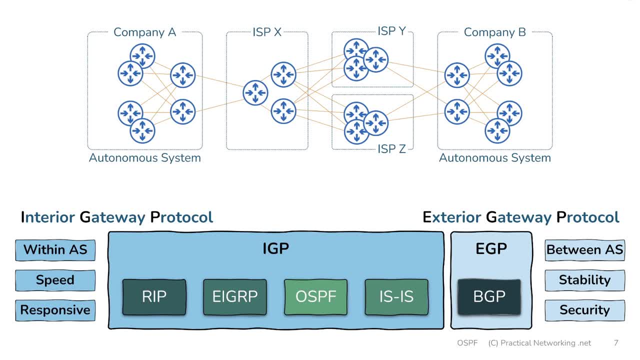 mention something in the comments below. Either way, BGP allows for all sorts of mechanisms for controlling the inbound and outbound paths between all these autonomous systems. BGP only offers a few ways to influence the path selection, which is another important difference between IGPs and EGPs. 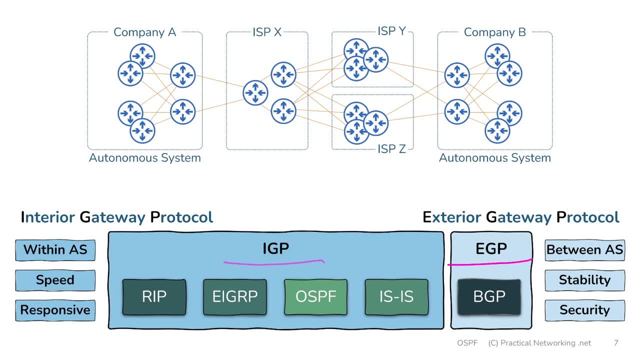 In any case, that's a high-level comparison of IGPs versus EGPs. The important thing, as a network engineer, is for you to understand the pros and cons of both and to make the best decision for your particular topology Either way. that's all we're going to speak about insofar as IGPs and EGPs. 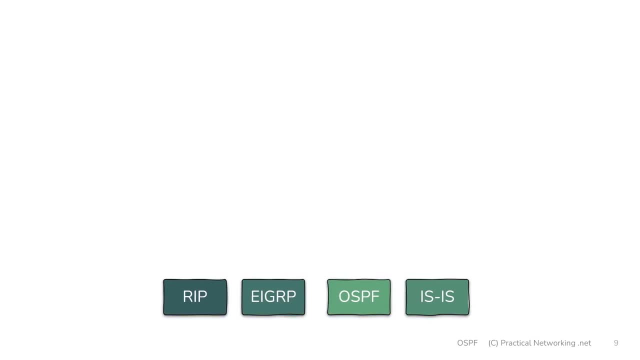 Next, we're going to dive a little bit further into these IGPs and break up these four protocols into two other categories: Distance Vector Protocol, which include RIP and EIGRP, and Link State Protocols, which include OSPF and ISIS. 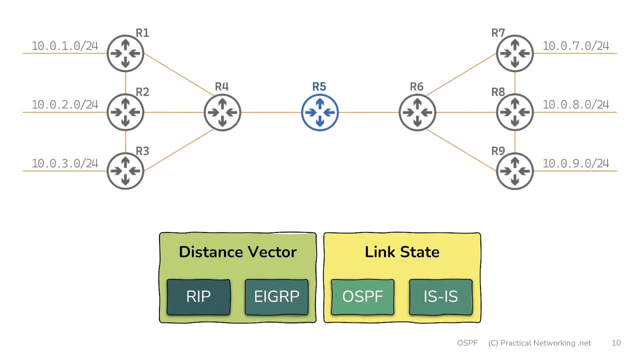 To talk about them. we're going to use this topology And we're going to start with Link State Protocols. A Link State Dynamic Routing Protocol is going to have knowledge of the entire network topology. So if all of these routers were doing a Link State Dynamic Routing Protocol with each other, 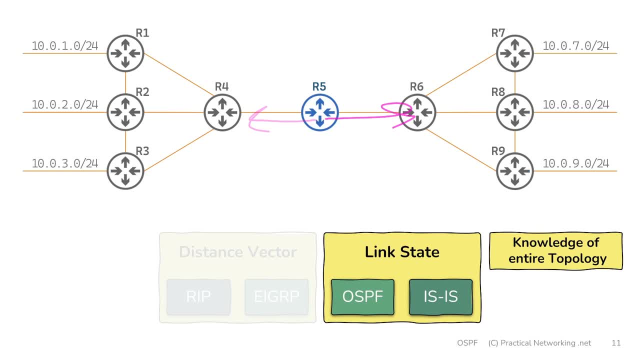 router 5 would know that it's connected to router 4 and router 6.. Router 5 would also know that router 6 is connected to router 7,, router 8 and router 9, and that router 7 and 8 are connected and router 8 and 9 are connected. 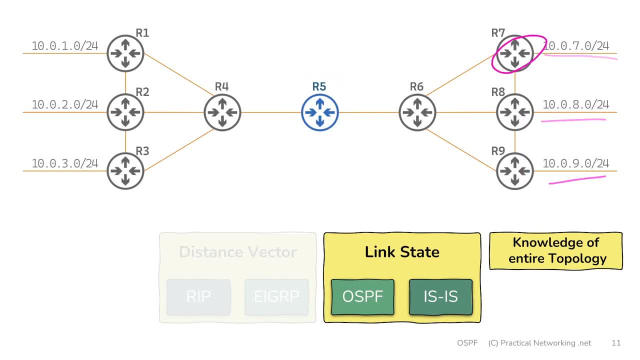 and router 5 would also know the three networks that are hanging off of router 7,, router 8, and router 9, and the same thing on the other side. Router 5 would know everything that's going on on that particular network. 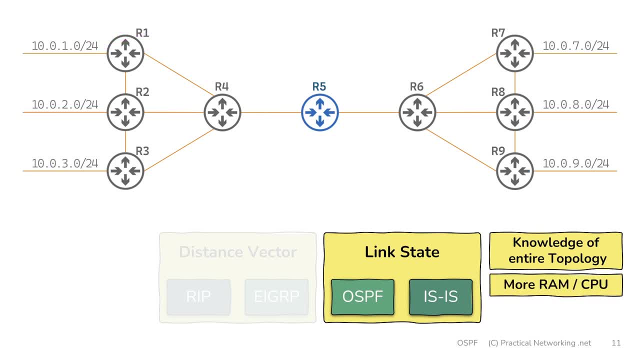 Now the price of all that additional knowledge is that it's going to cost more ram and cpu resources to maintain the knowledge of the entire topology. is that Router5 will be better equipped to converge in case there's some sort of failure event. Link state protocols typically have faster conversions. 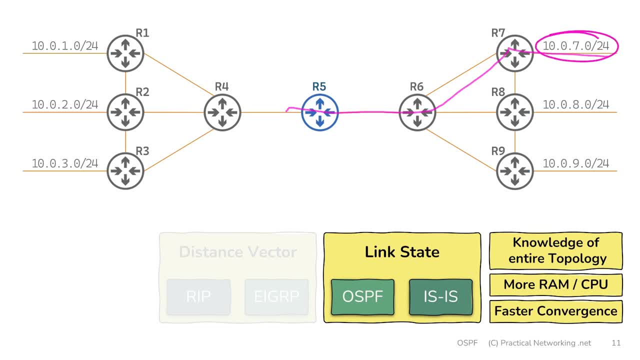 What I mean by that is if Router5 is taking this path to get to the 10.0.7.0 network and something happens to this link, well, Router5 already knows of a second path to get to that particular network, So there's nothing new that Router5 has to learn. 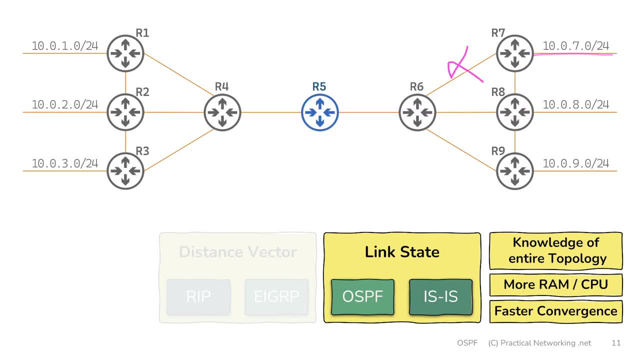 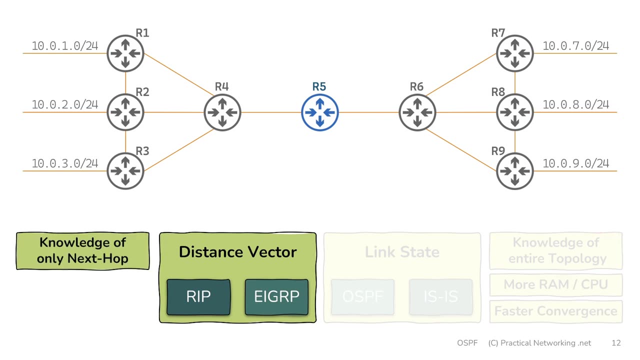 It already knows how to get here if something were to happen to that link. So that's a rundown of link state protocols, Which now brings us to distance vector protocols. Distance vector protocols, unlike link state protocols, only have knowledge up to the next hop. 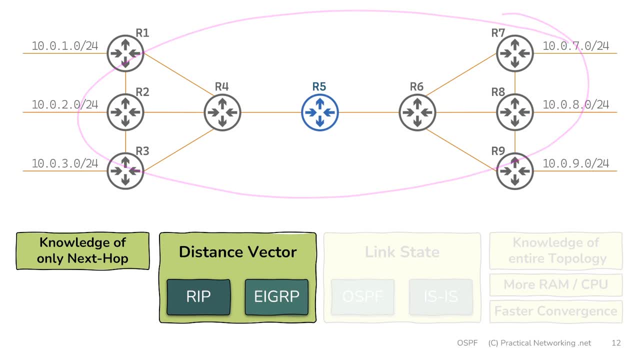 So if all of these routers were doing a distance vector dynamic routing protocol with each other, Router5 would know it's connected to Router4 and to Router6, but wouldn't know anything happening on the other side of Router4 or Router6. Router5 would simply know that these three networks 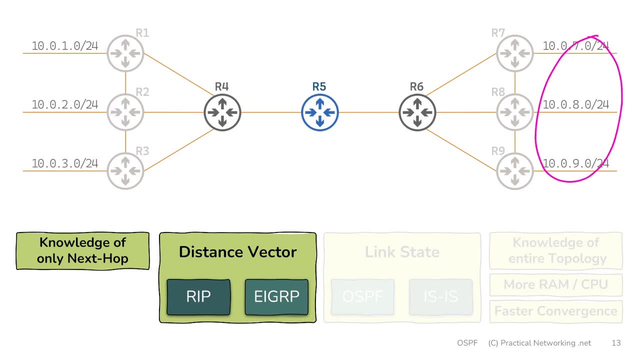 exist on the other side of Router4, and these three networks exist on the other side of Router6. But Router5 would have no knowledge about Router7,, 8, and 9, or 1,, 2, and 3.. 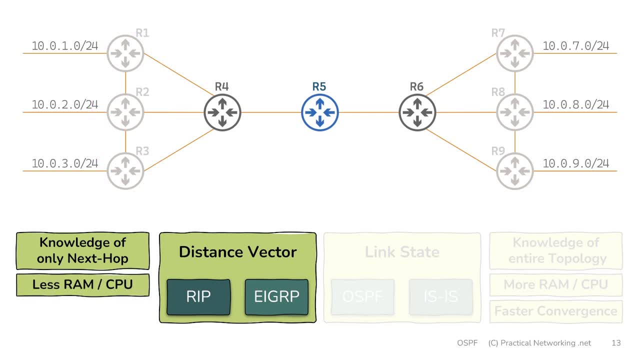 The benefit to that is that Router5 wouldn't have to spend as much resources to maintain knowledge of the networks that exist in this topology. But the cost of that is that distance vector protocols typically converge a little bit slower. They're also slower to react to some failure events. 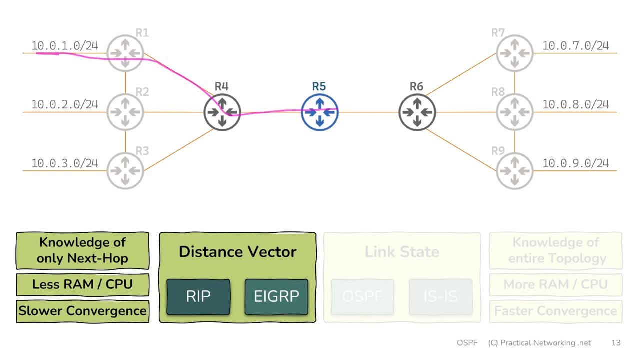 Meaning if Router5 is taking this path to get to the 10, 0, 1 network. if something were to happen to that link, Router4 might tell Router5 that it no longer has access to the 10, 0, 1 network. 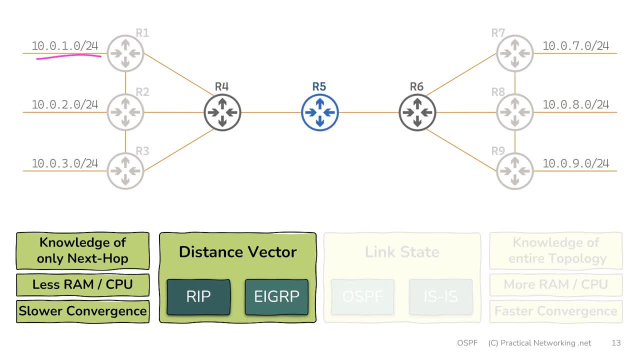 And Router5 will now have zero paths to get to the 10, 0, 1 network. It won't regain access to that network until Router1 tells Router2 that it can still reach the 10, 0, 1 network. 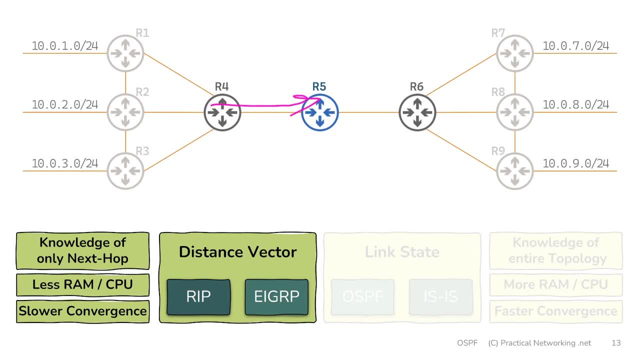 and Router2 passes that on to Router4, and then Router4 again passes that on to Router5 that it can now reach the 10, 0, 1 network. But throughout that time Router5 will have no connectivity to the 10, 0, 1 network. 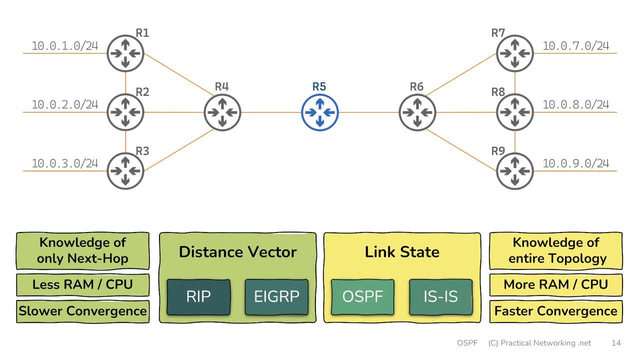 That's the rundown on distance vector protocols and link state protocols And again, it isn't that one is better than the other. It's that both of them have different pros and cons and it's up to you to make the best decision about which you want to use in your particular network. 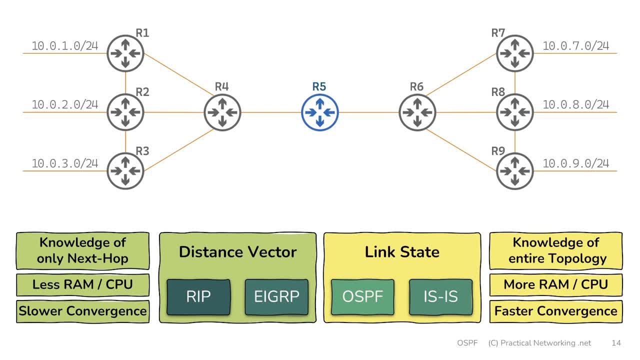 If you're using older devices and a somewhat simplistic topology, then maybe you can get away with using a distance vector protocol. But if you're using more modern gear and you have a topology that highly prioritize redundancy, then maybe you ought to do something like a link state protocol. 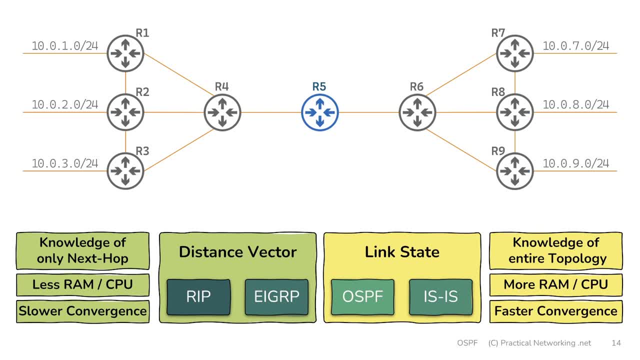 Now, since we're in 2022, as I'm recording this, I do want to quickly mention that the cost of more RAM and more CPU on today's modern routers are largely inconsequential. Consider that most of these protocols were written back in the mid 90s and in those days. 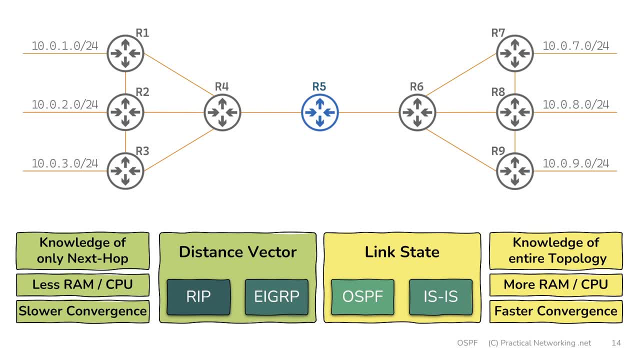 routers had something like 64 KB RAM or 128 or 256 KB RAM, And so whatever additional RAM link state protocols required was actually relatively more costly Nowadays. any router built in the last 10 years is probably going to have enough memory to have 10,000 or even 100,000 routes. 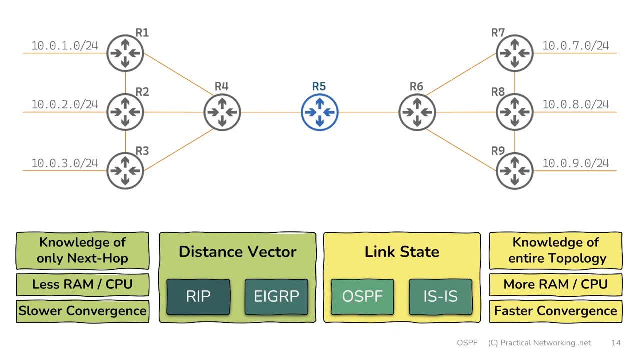 in a link state database And it's going to be able to handle that just fine. And finally, the last thing I'll mention on this particular slide is, while EIGRP is typically considered a distance vector protocol, it's sometimes considered a hybrid protocol. 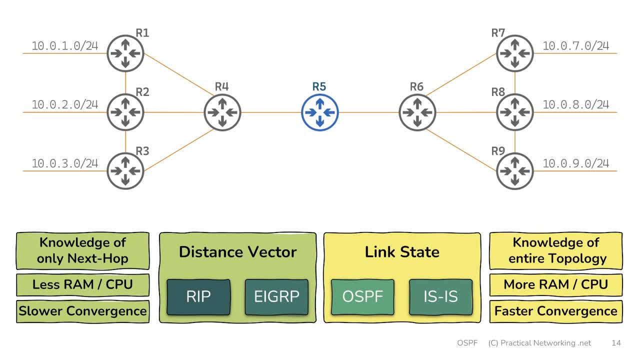 or even an advanced distance vector protocol, because it includes certain features that only exist in link state protocols. So it does a little bit of both. One in particular is very eager to tell you that EIGRP is an advanced distance vector protocol, to put the protocol that they invented in a better light. 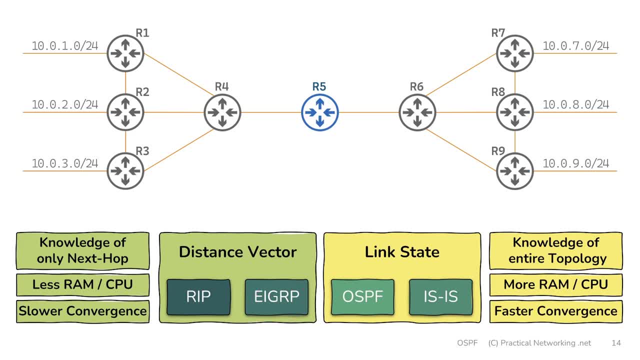 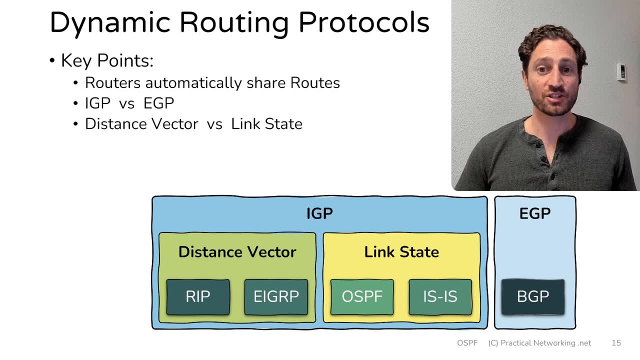 Either way, that's all I wanted to communicate to you about distance vector protocols and link state protocols, And that actually wraps up this lesson. The main takeaways from this lesson is understanding that a dynamic routing protocol allows routers to automatically share routes with another. 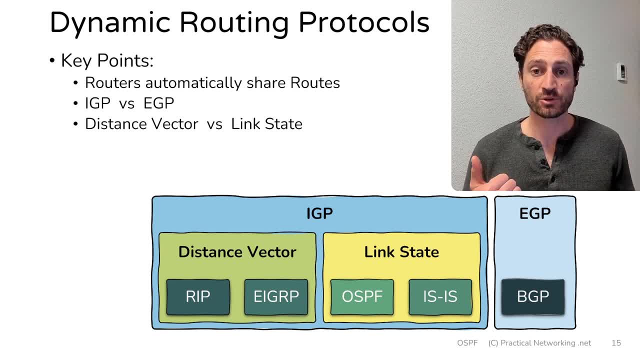 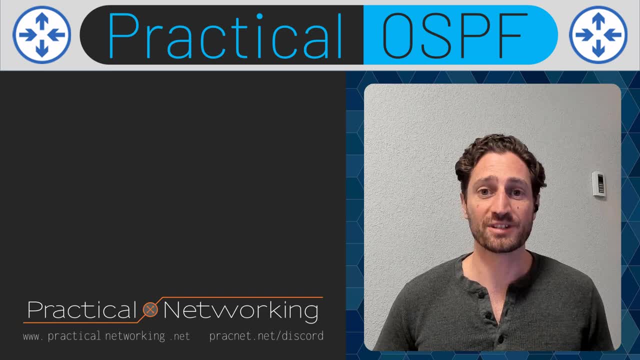 and understanding the two categories that we discussed: interior gateway protocols versus exterior gateway protocols and distance vector protocols versus link state protocols. If you enjoyed this lesson and think it should be shown to a wider audience, you can help me out by hitting the like button.